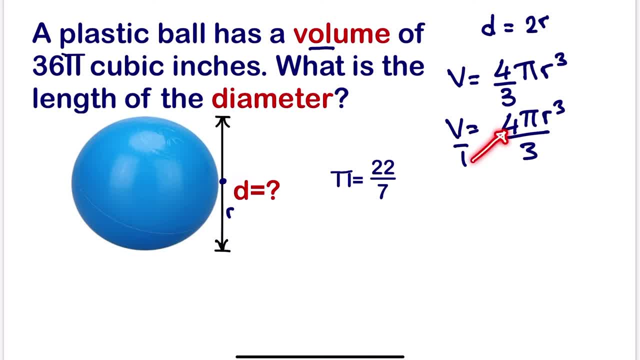 fraction. So if we cross, we can cross multiply, this time this and this time this. So we are going to have 1 times 4 pi r squared will be 4 pi r cubed. sorry, should be equals to 3 v, 3 times 3, 3 times 3 if we cross multiply. 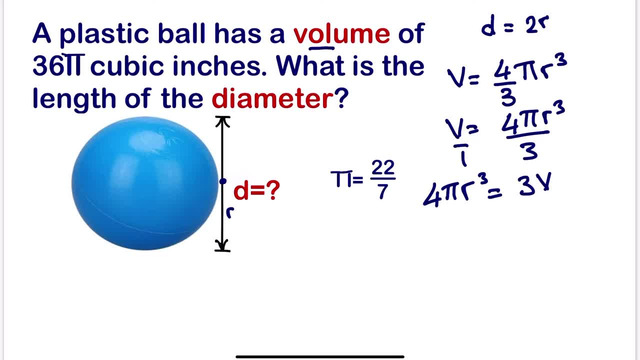 Okay, so next we can as well make r cubed the subject, So r cubed will be the same as. remember: if you have 2x equals to 10, you want to make x a subject, So you need to divide by the coefficient of x. So x is the same as 10 divided by 2.. So we are going. 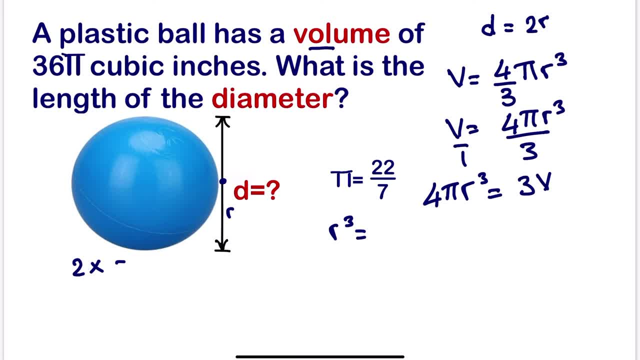 to apply that here in solving further radius. So we want to make r cubed the subject. So we are going to have r cubed will be equals to 3 v divided by 4 pi. Okay, so if we move further, we are going to substitute now the value 3 v. 3 v would be the same as 4 pi. 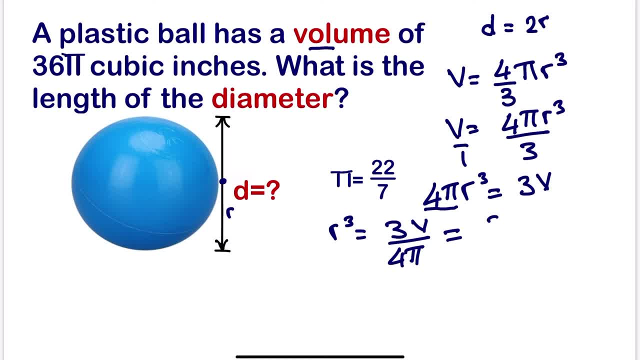 So if we move further, we are going to substitute now the value 3v. 3v would be the same as 4 pi times the volume is 36 pi divided by 4 pi. so we can see that pi and pi we can. 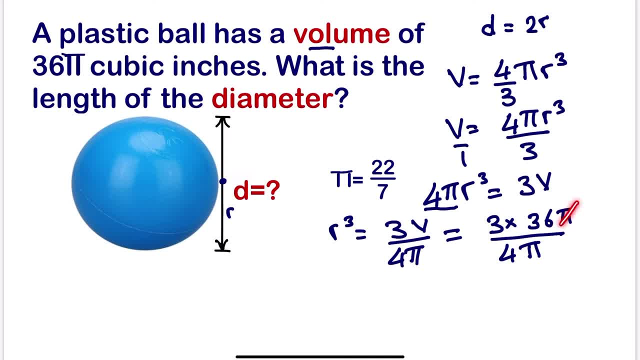 simplify. so pi will divide. pi will be left with this. so we can also divide 4 divided by 36. so pi divided by pi will cancel. up will be left with. we can divide: 4 divided by 36 is 9. so our cube will be equals to 3 times 9, which is 27.